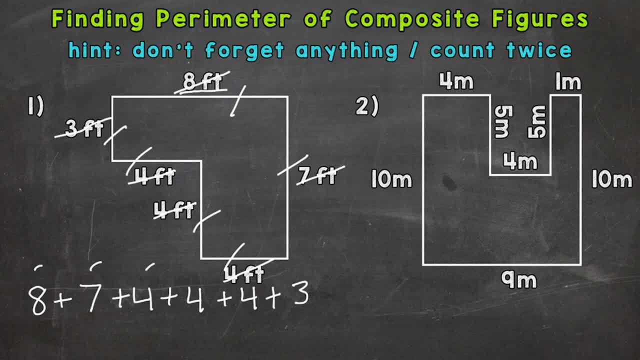 six sides And we have one, two, 3, 4, 5, 6 measurements down there that we are adding up. so we're good to go. let's add: 8 plus 7 is 15, plus 4 is 19, plus another 4 is 23, plus another 4 is 27 plus 3 gives us 30, and this is feet. 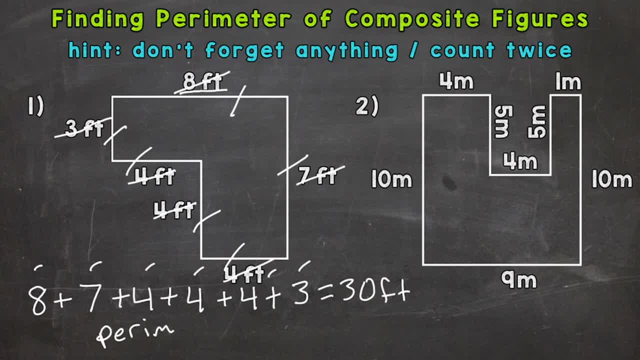 so down below I'll put our final answer: perimeter equals 30 feet. we can circle our final answer there and let's move to number two. now this figure has more sides than number one, so again, we are going to have to be careful and organized as we go through our figure and the side measurements. 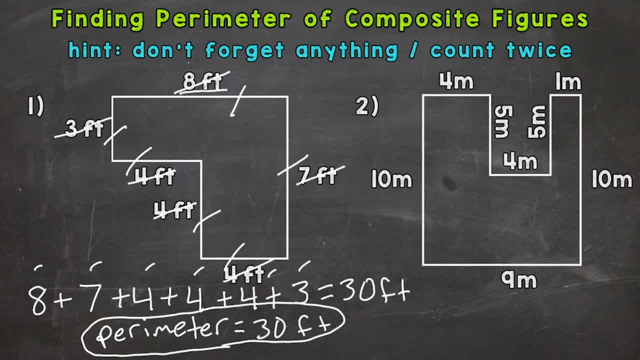 so we'll start up top with the four meters here, and before I start, it doesn't matter whether we're going to be able to do this or not. we're going to have to be careful which side or measurement you start with. I usually just like to start up top, but really 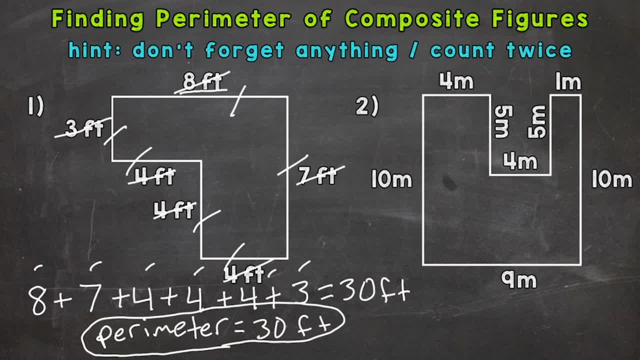 it doesn't matter. so the other strategy. if you don't like crossing out off, you can circle the numbers as you go along. same, same idea here. so 4 plus 5 plus 4 plus 5 plus 1 plus 10. I'm running out of room, so I'm going to go to the next line here, plus 9 plus 10, and let's. 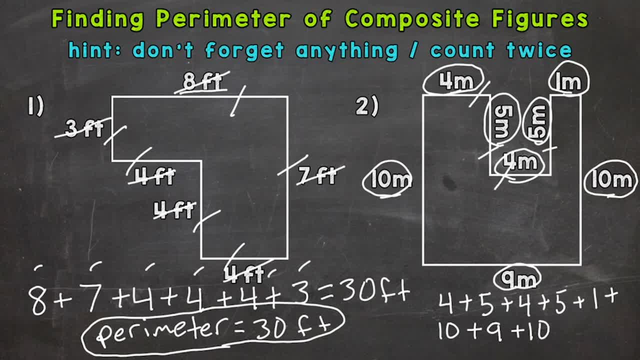 double check everything. we have one, two, three, four, five, six, seven, eight sides, and we have one, two, three, four, five, six, seven, eight measurements. let's add them up so we have: four plus five is 19 plus 4 is 13, plus 5 is 18, plus 1 is 19 plus 10 is 29 plus 9 is 38 plus another 10 is 48, so our 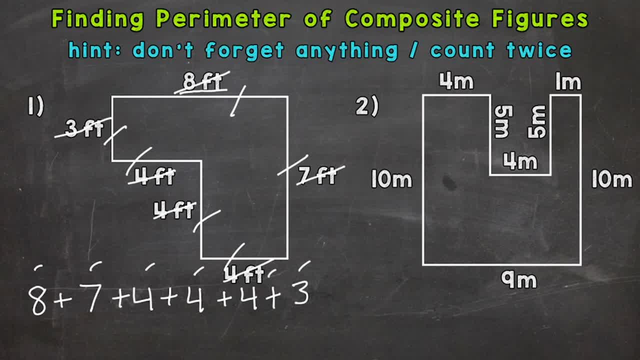 two, three, four, five. So I've got two here and six pieces of this, And this is the height at which 3,, 4,, 5, 6 measurements down there that we are adding up. So we're good to go. 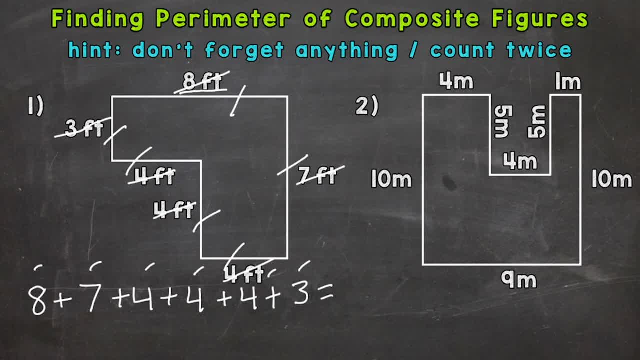 Let's add 8 plus 7 is 15,, plus 4 is 19,, plus another 4 is 23,, plus another 4 is 27,, plus 3 gives us 30, and this is feet. So down below I'll put our final answer: perimeter equals 30 feet. 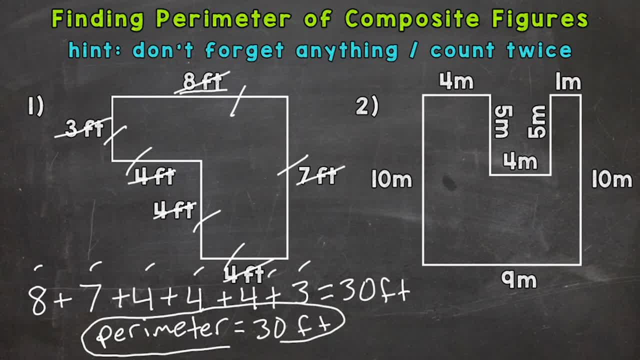 We can circle our final answer there And let's move to number 2.. Now this figure has more sides than number 1, so again, we are going to have to be careful and organized as we go through our figure and the side measurements. 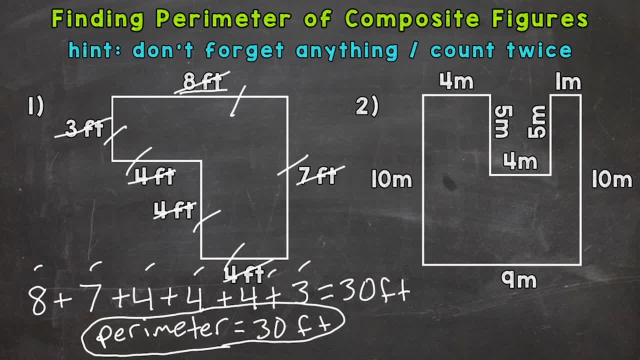 So we'll start up top with the 4 meters here. And before I start, it doesn't matter which side or measurement you start with. I usually just like to start up top, but really it doesn't matter. So the other strategy: if you don't like crossing off, you can circle the numbers as you go. 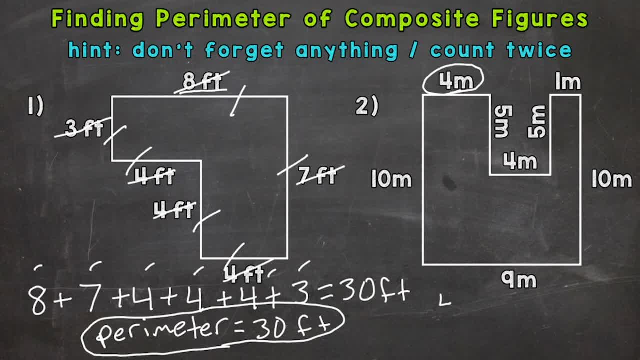 along Same idea here, So 4 plus 5 plus 4 plus 5 plus 1 plus 10.. I'm running out of room, so I'm going to go to the next line here: Plus 9 plus 10.. 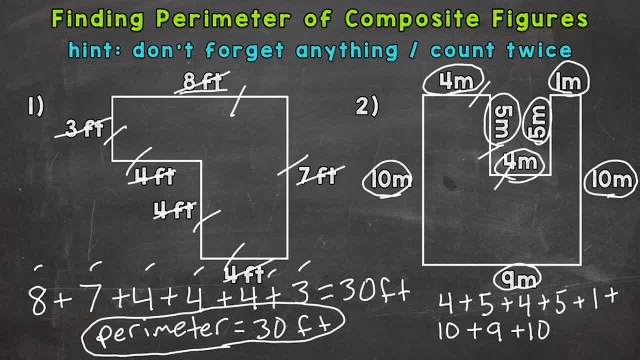 And let's double check everything. We have 1,, 2,, 3,, 4,, 5,, 6,, 7, 8 sides and we have 1,, 2,, 3,, 4,, 5,, 6,, 7,, 8 measurements. 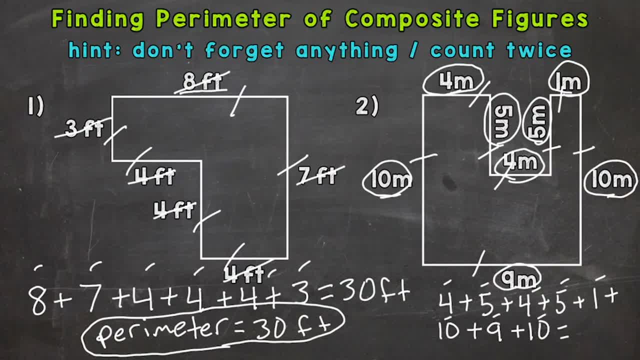 Let's add them up, So we have: 4 plus 5 is 9, plus 4 is 13, plus 5 is 18, plus 1 is 19, plus 10.. Here we are, Let's get our measurement.